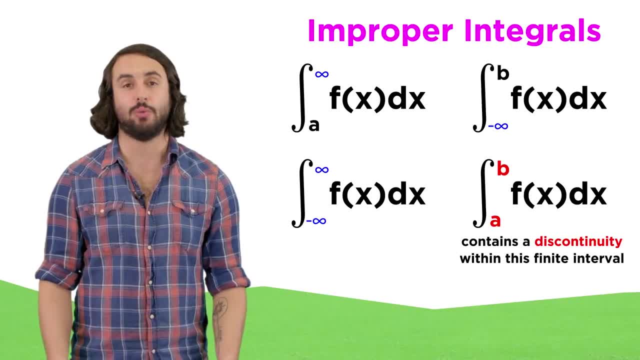 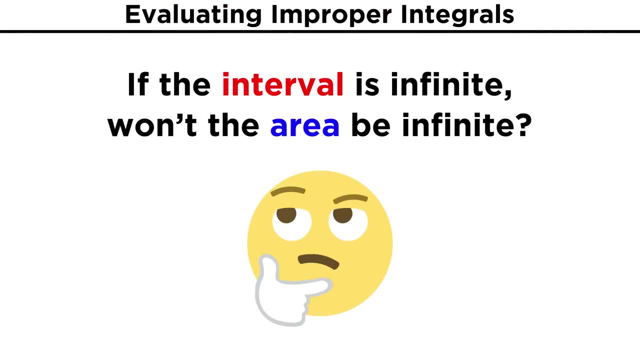 When this is the case, we call these improper integrals. Let's learn about these now. Now, one might initially assume that if the interval is infinite, the area under the curve must also be infinite, But actually this is not always the case. 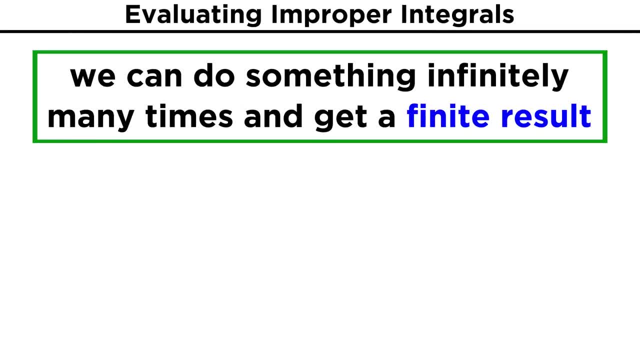 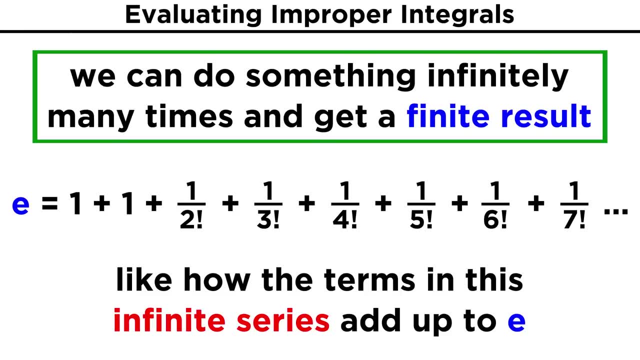 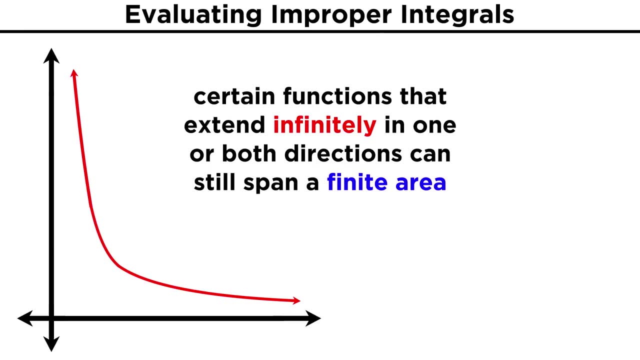 We've seen countless times by now that calculus is all about doing something infinitely many times and getting a finite result, kind of like the infinite series that sums to give E. So we can indeed have a function that extends infinitely in a particular direction, and 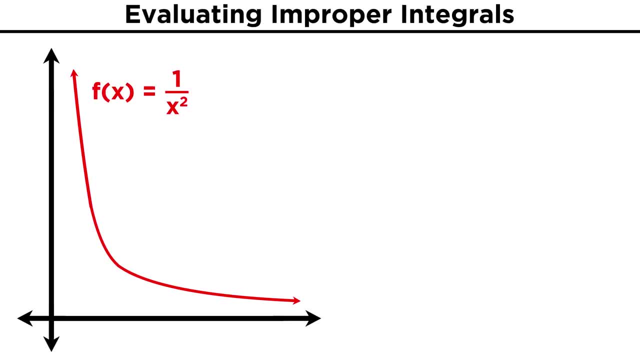 yet spans a finite area. Take, for example, the curve one over x squared. Let's say we want to integrate this, starting at x equals one and going to infinity. To examine what happens as we get closer to infinity, let's select an arbitrary upper. 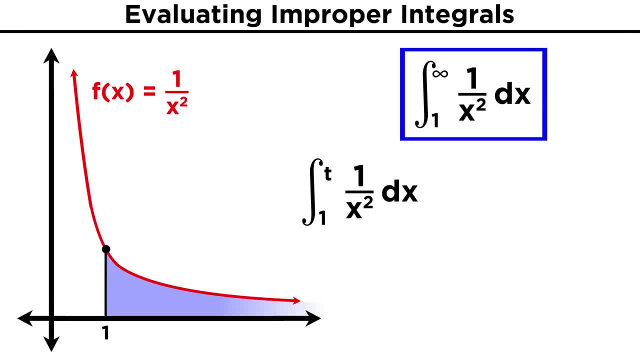 limit of integration and call it t. We can treat this like a definite integral and get the antiderivative X to the negative. two will give us x to the negative, one over negative one, which is negative one over x. Let's evaluate this over our selected interval and we get negative one over t, minus negative. 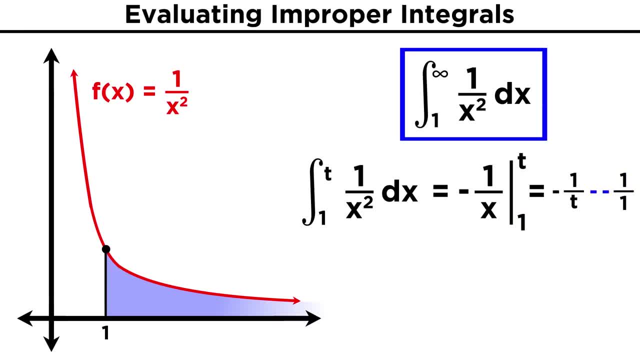 one over one. These two negative signs cancel to give us positive one and switching the order, we can express this as one minus one, So we get negative one over t minus negative one over one. So if we take t to equal two, we get one minus one half, which is one half. 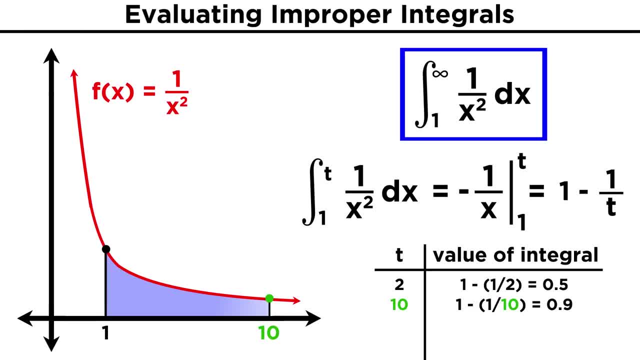 If we take t to equal ten, we get one minus one tenth or nine tenths. We can plug in larger and larger values for t and we get closer and closer to one. and if we plug in infinity for t, which is one minus one tenth, we get one minus one tenth. 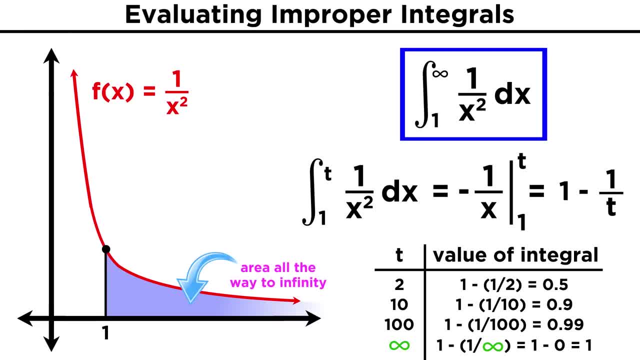 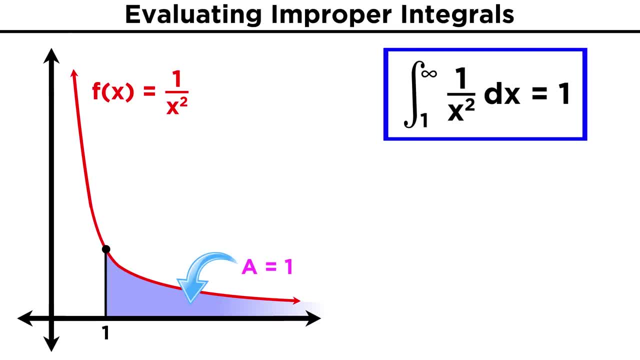 or nine tenths, Which means integrating over this whole portion of the function all the way to infinity. then we get one as the answer. That means, quite incredibly, that the area under the curve from x equals one. all the way to infinity is one. 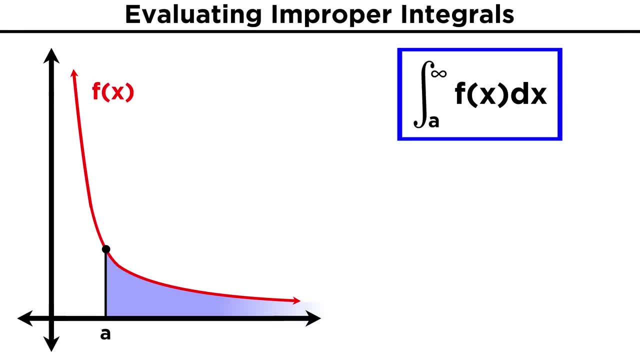 This gives us a simple way to evaluate improper integrals. We can integrate f of x, dx from a to infinity, and this will simply be equal to t, to the negative one over t, minus negative one over one, To the integral over the definite interval from a to t in the limit of t approaching. 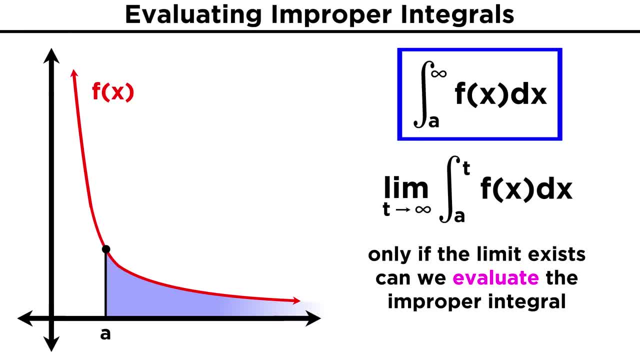 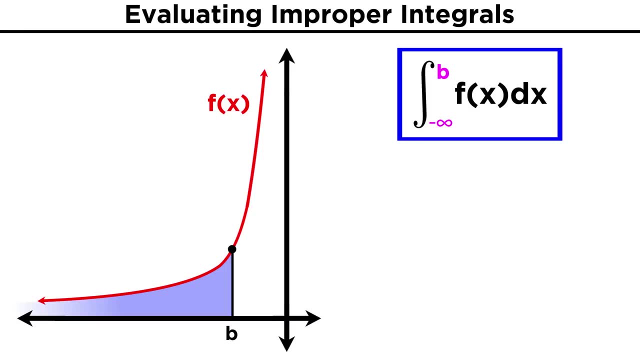 infinity. This limit may or may not exist, which means that not all improper integrals can be evaluated, but some indeed can. This also works in the negative direction. If we are integrating from negative infinity to b, we just integrate from t to b and see. 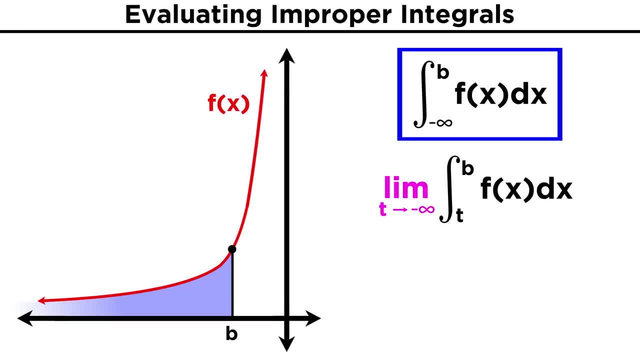 what happens in the limit of t approaching negative infinity. So we can see that the integral over the definite interval from a to t in the limit of t to infinity is one If we are evaluating an improper integral and we do get a finite number as an answer. 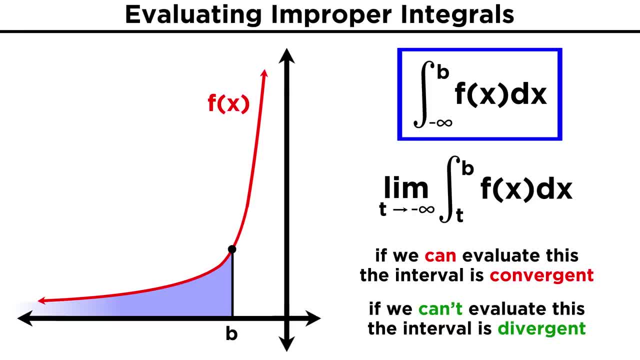 then we say that the interval is convergent. If the limit does not exist, meaning the area truly is infinite, we say that the interval is divergent. Unfortunately, it may be difficult to tell whether an integral is convergent or divergent. 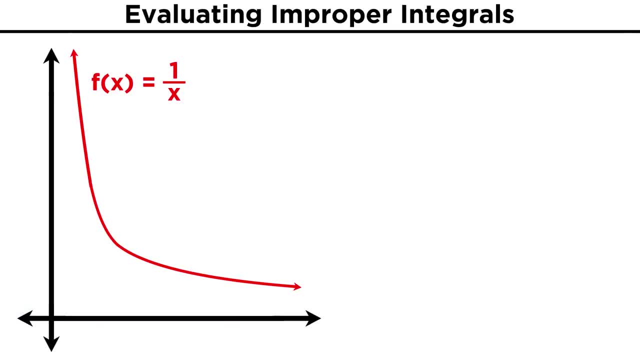 just by looking at it. Say, we tried to do the same thing when we did the same thing. What would happen if we tried to do the same thing when we did the same thing with one over x? We can integrate this function from one to infinity by replacing infinity with t. 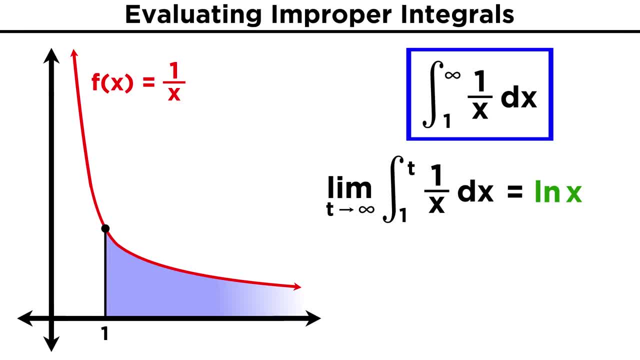 The integral of one over x is the natural log of x. so when we evaluate we get the natural log of t minus the natural log of one. The natural log of one or any log of one must be zero, because anything to the zero 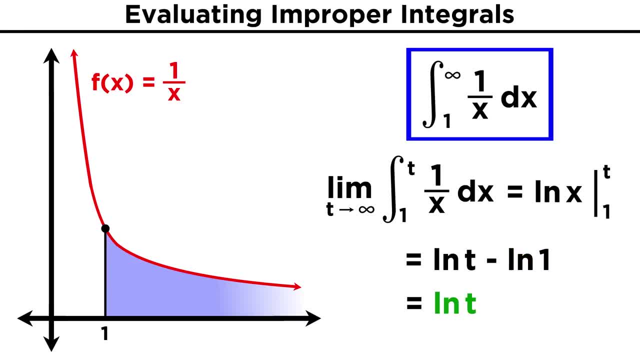 power gives us one. So that term goes away, leaving us with the natural log of t. As t gets larger, this term gets larger, and it does so without bound, all the way to infinity. So this one didn't work out as nicely as the first one, and this integral is indeed. 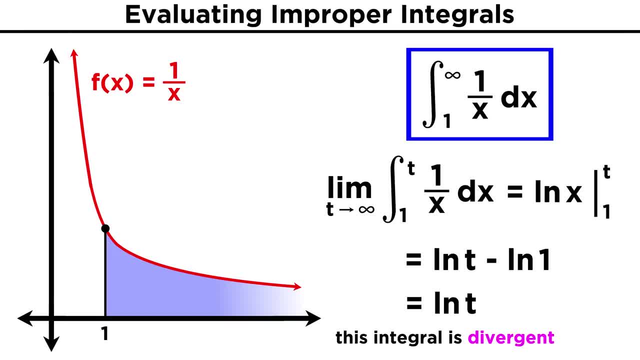 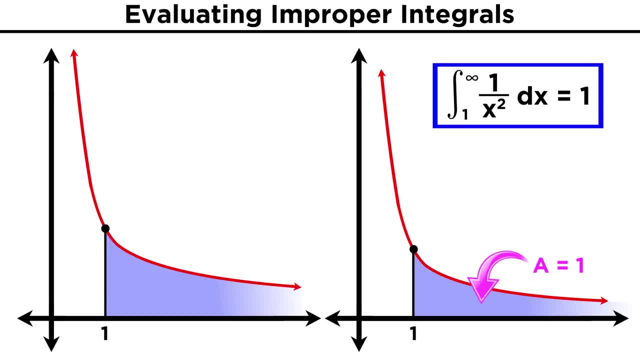 divergent, even though the two functions look fairly similar. From this we conclude that one over x squared gets small enough fast enough that the area under the curve is finite, While one over x is small enough that the area under the curve is finite. 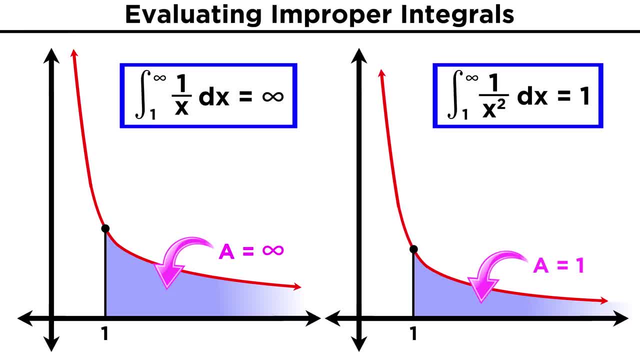 While one over x is small enough that the area under the curve is finite, While one over x also gets small enough, as it too goes to zero as x approaches infinity. it just doesn't do it fast enough, and we needed calculus to tell us this fact. 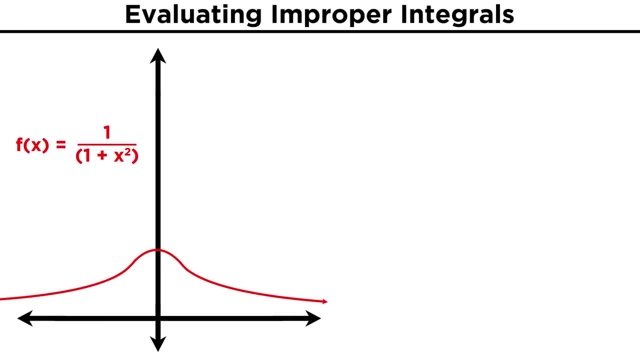 Let's try another one. How about one over the quantity one plus x squared? This function looks like this, extending to positive and negative infinity in either direction, and it's perfectly symmetrical. so let's just pick one half. How about from zero to infinity? 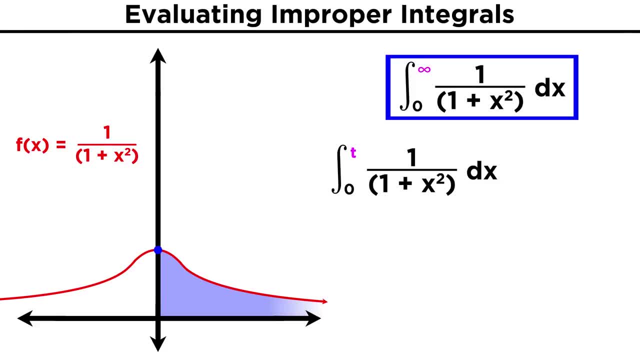 How about from zero to positive infinity? So, as we know, we change infinity to t and we integrate. If we consult our table of common integrals, this is actually a special one as it fits the form of one over x squared plus a squared, and in this case a equals one. so we get: 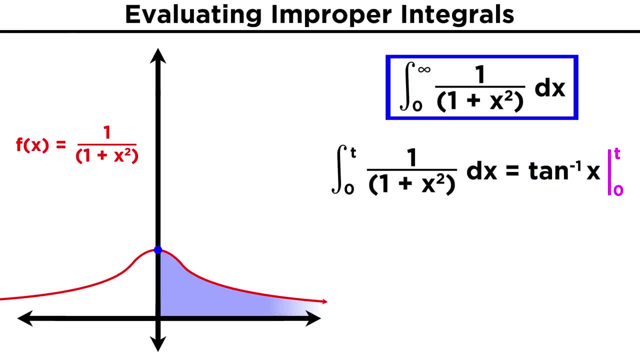 inverse tangent of x. We will then evaluate this at t and then zero, and we get inverse tangent of t minus inverse tangent of zero. We can evaluate the inverse tangent of zero quite easily. It is simply the angle that gives us a tangent value of zero. 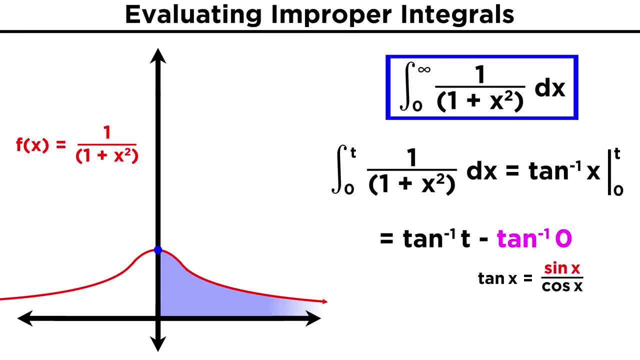 As tangent is sine over cosine. when sine is zero we get zero overall and sine is zero at zero. so inverse tangent of zero is zero. That leaves us with the inverse tangent of t, which we must now examine as t approaches infinity. 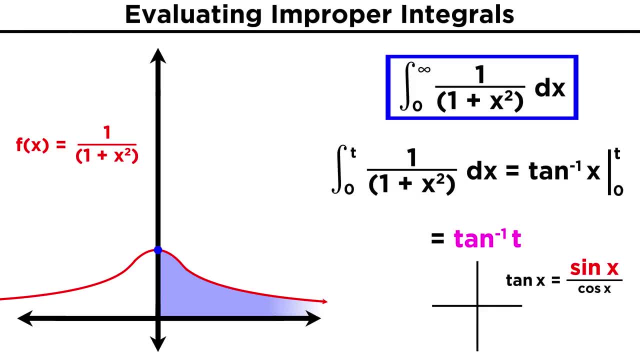 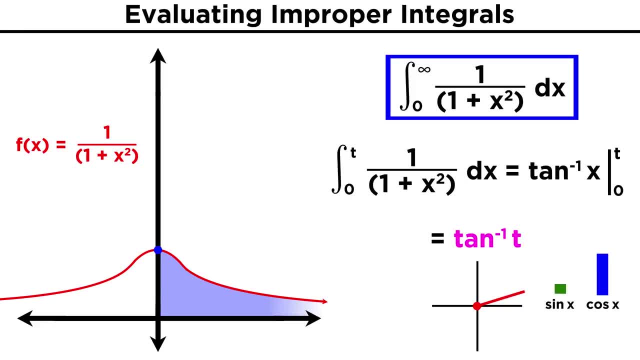 infinity. Moving through quadrant one, the tangent value approaches infinity until we get to half pi, where it is undefined. That means that the inverse tangent of infinity is half pi. So the area under this half of the curve is half pi. To get the other half, we could do the exact same thing, but integrate from t to zero. 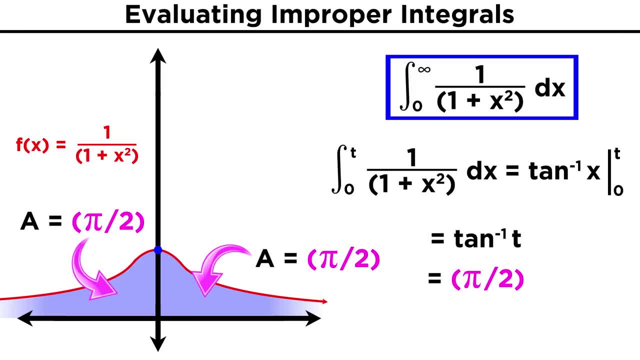 and we would again get half pi, which makes sense as this is perfectly symmetrical, and half pi plus half pi is pi. So the area under this entire curve, which spans from negative infinity to positive infinity, is actually a finite number. pi and this integral, no matter what the interval is. 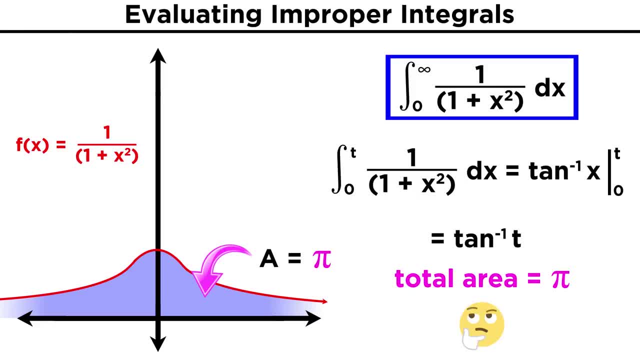 indeed convergent. So let's look at this again, Let's look at this again. Let's look at this again. If the integral from negative infinity to positive infinity yields a finite number, we might also be quite astonished that this number is pi. 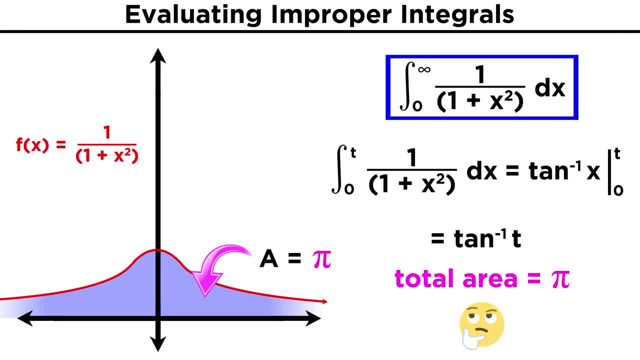 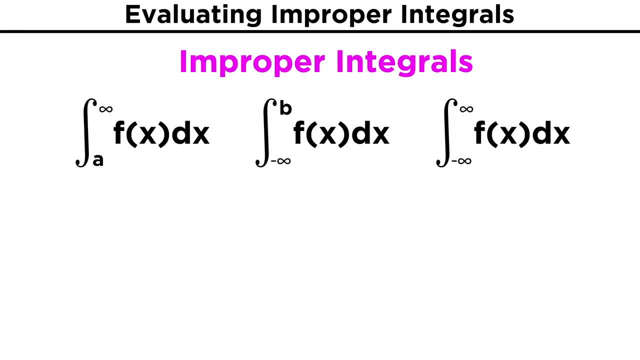 We are used to seeing pi when dealing with circles, and here there is no circle to be found, just another example of the stunning beauty and mystery that can be found in mathematics. So integrating over an infinite interval is one way we can get an improper integral. 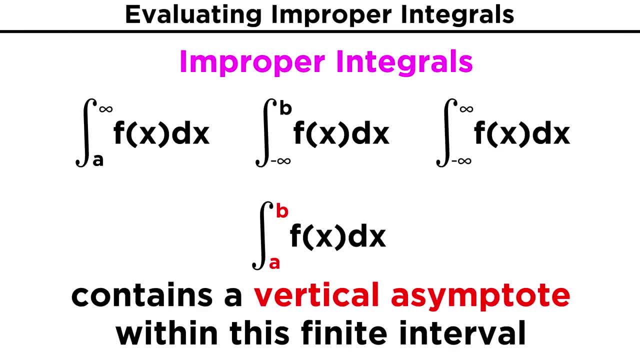 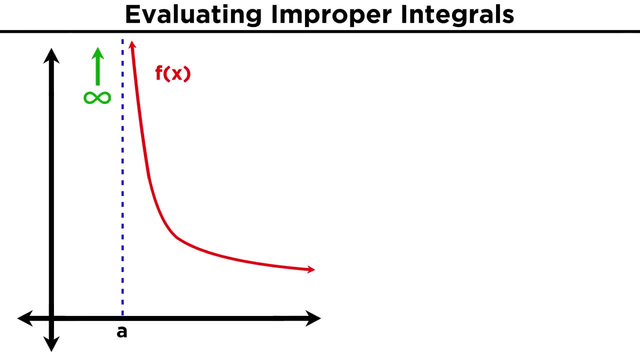 There is another way that involves finite intervals, And this will be when there is some vertical asymptote within the interval. This allows the curve to extend to infinity, not in the horizontal direction, but in the vertical direction, and we might not be too surprised by now to find out that this circumstance 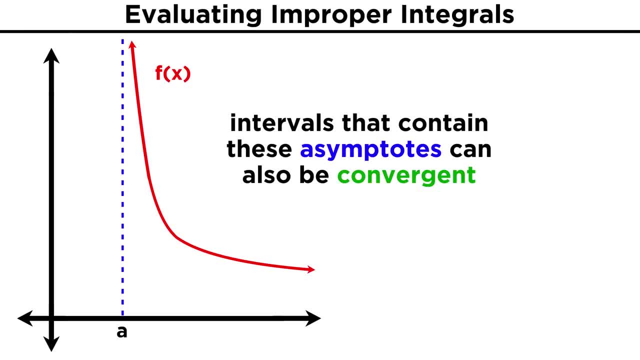 can also yield a convergent integral with a finite value To evaluate these. it's not much different. It's just that, instead of replacing infinity with t, we replace either one of the limits of integration, If one of the limits is the asymptote. 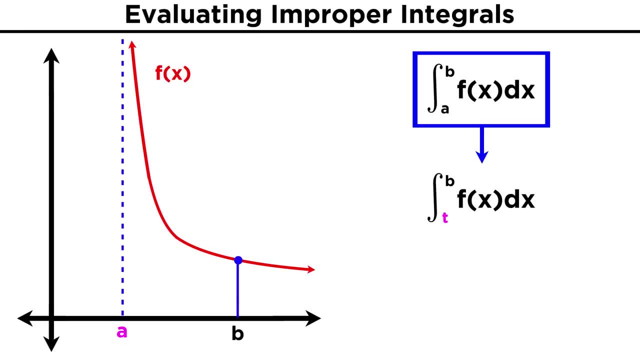 If one of the limits is the asymptote Or we replace some value in between with t. if the asymptote is in the middle of the interval, Let's take the function one over root x minus two and integrate from two to five. 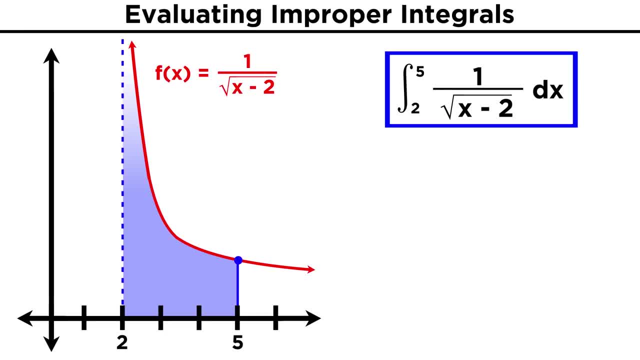 This function has a vertical asymptote at x equals two, so we can see that this will be an improper integral. So instead of integrating from two, we have to integrate from t, and then look at what happens to the integral as t approaches two from the positive direction. 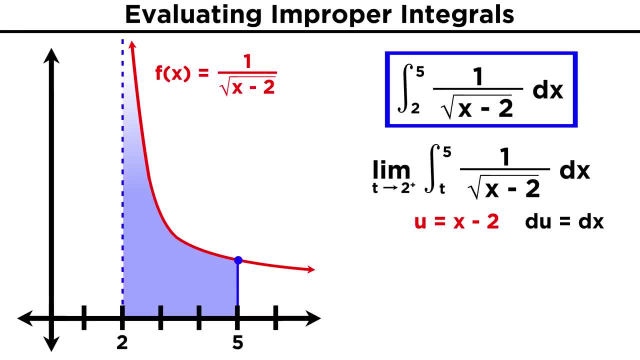 To integrate. let's just use a simple substitution, changing x minus two into u. That means that du will be equal to dx and we have u to the negative, one half du. Integrating will give us u to the positive one half, over one half or two root u. 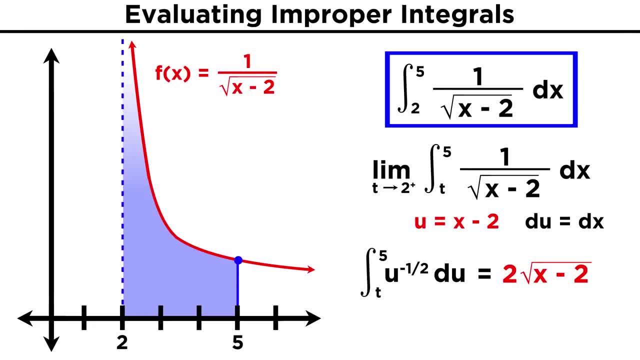 We then change u back and we have two root x minus two. Let's evaluate this at five and t For four. we have two root x minus two, and we have two root x minus two. Let's evaluate this at five and t For four. we have two root x minus two. 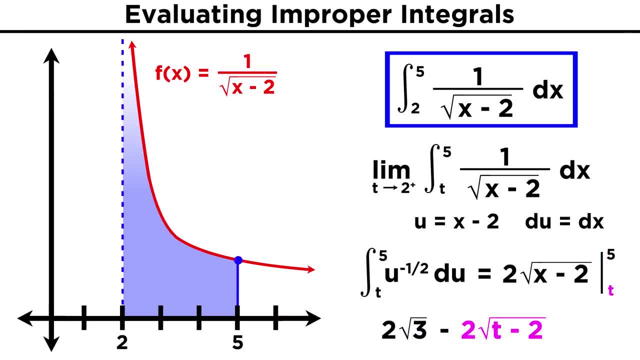 For five, we get two root three and for t, we get two root t minus two. As t approaches two from the positive direction. what's inside? this radical remains positive but gets closer and closer to zero and in the limit of t, approaching two this term. 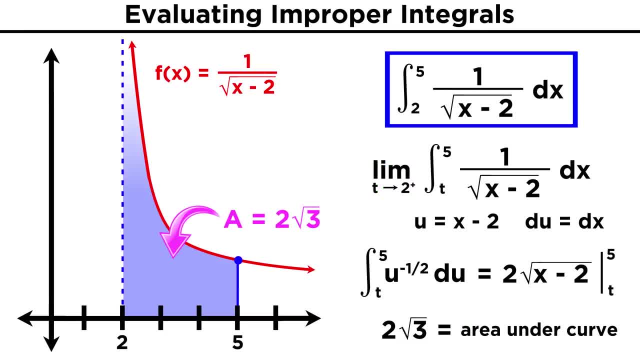 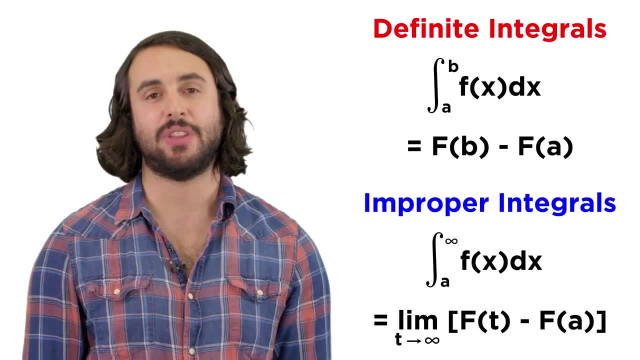 will become zero. So the answer is two root three for the area under the curve for this interval, and the integral is therefore convergent. So we can see that evaluating improper integrals is not that much different than evaluating regular, definite integrals. 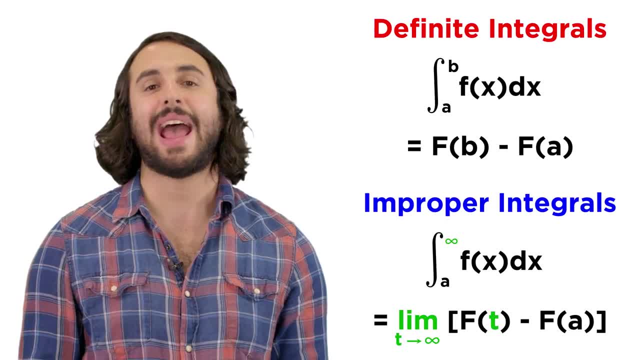 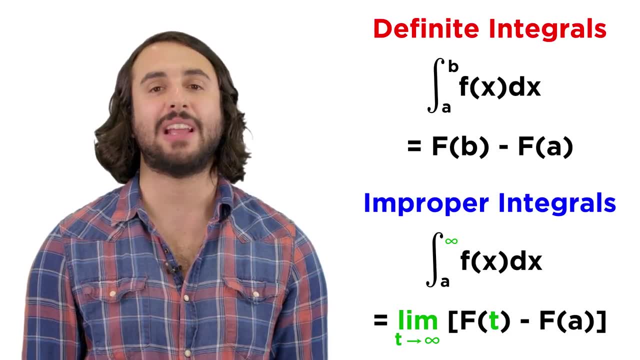 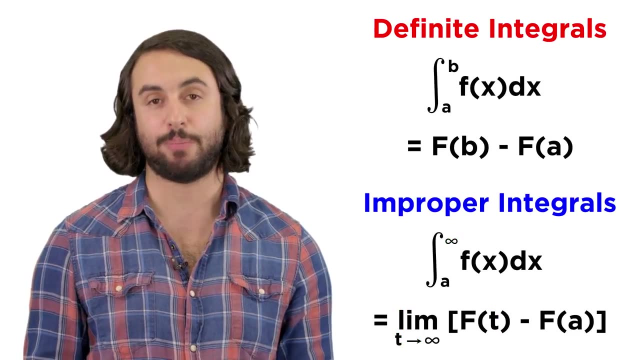 In fact it's exactly the same. it's just that we see what happens when one of the limits of integration starts moving towards some particular value, whether positive or negative, infinity or some vertical asymptote. It is very important to recognize when an integral is improper, because we must evaluate. 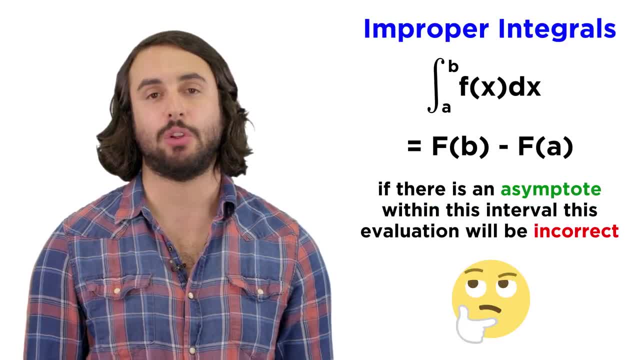 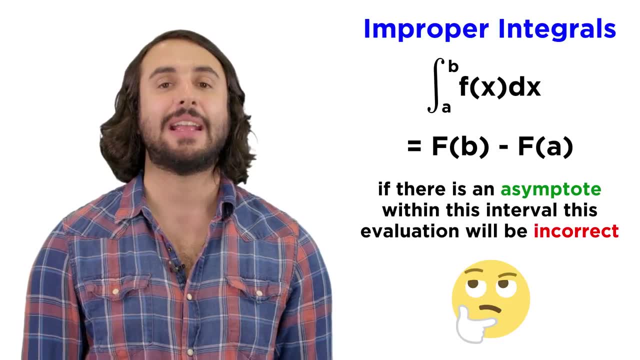 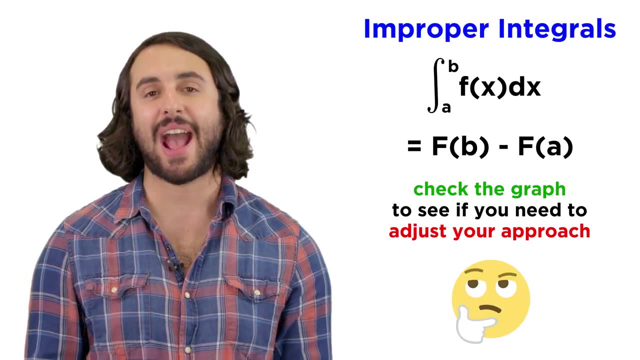 it accordingly. Evaluating an improper integral as though it is a definite integral, simply evaluating the antiderivative at the limits of integration and subtracting can indeed yield incorrect values. So as you go about integrating, if something looks like it might have an asymptote of some, 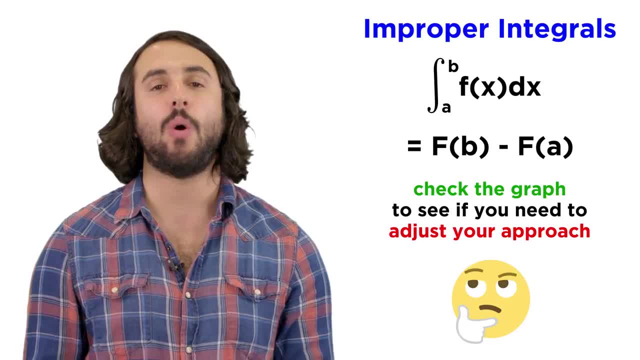 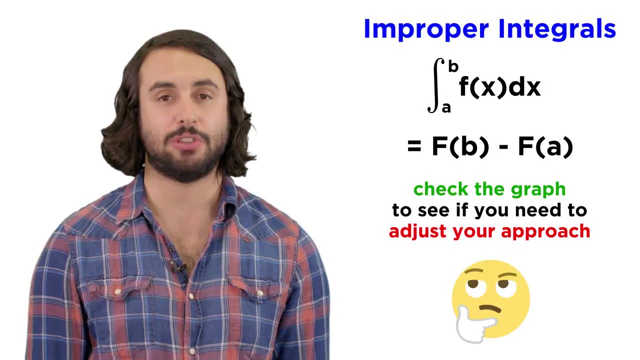 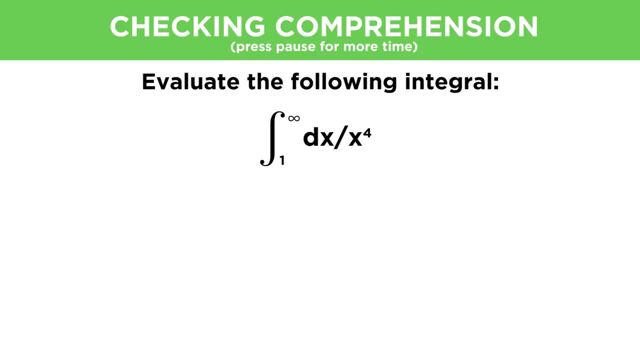 kind, check the graph of the function being integrated over the specified interval to see if you need to adjust your approach accordingly. With that understood, let's check comprehension. Thanks for watching, guys. See you next time, Bye, Bye, Bye. 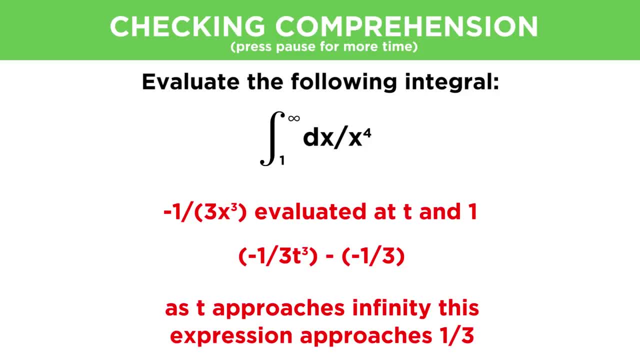 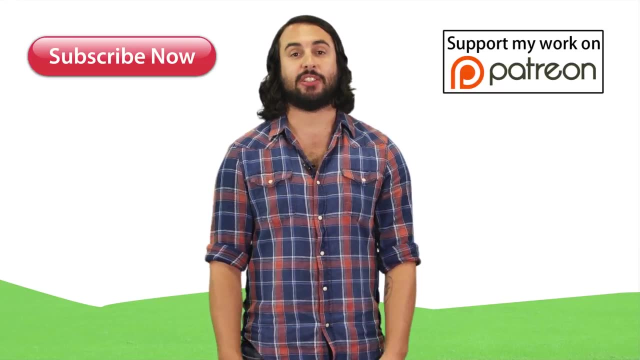